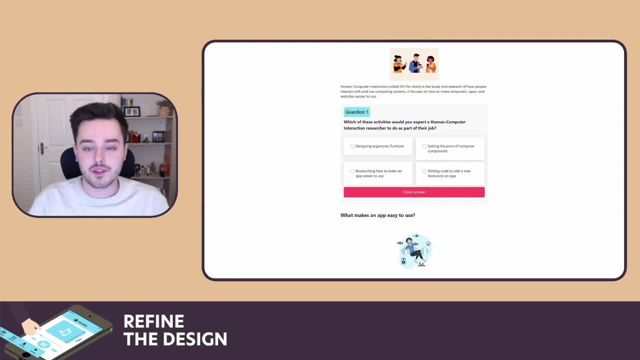 a study and research of how people interact and use computing systems. It focuses on how to make computers and apps and websites easier to use. That takes us on to question one: Which of these activities would we expect a human computer interaction researcher to do as part of their job? 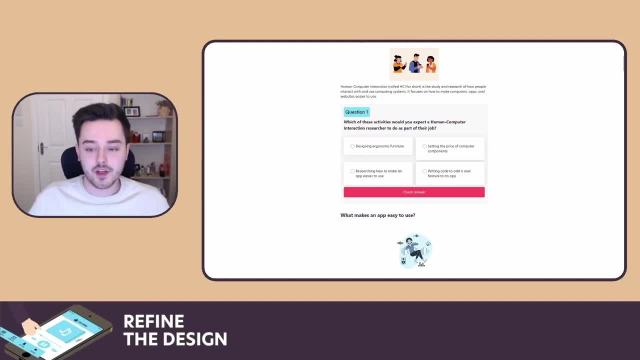 So the options we have are designing ergonomic furniture, setting the price of computer components, researching how to make an app easier to use and rating quotes at a new feature to an app. So I'm going to select this one here and press check my answer And that's the correct answer. 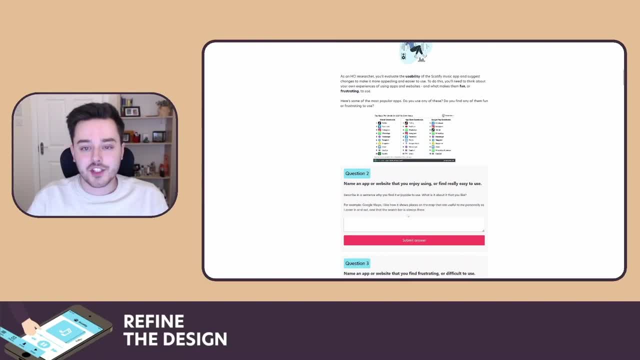 So what makes an app easy to use? The reheat CIFE searcher will evaluate the usability of the Scottify music app and suggest changes to make it more appealing and easier to use. To do this, we think of, about our own experiences of using apps and websites and what makes it fun or frustrating. 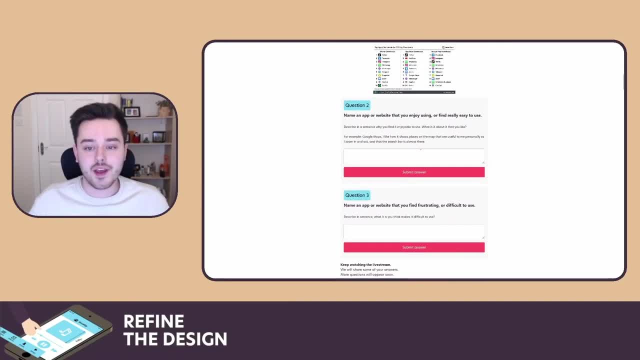 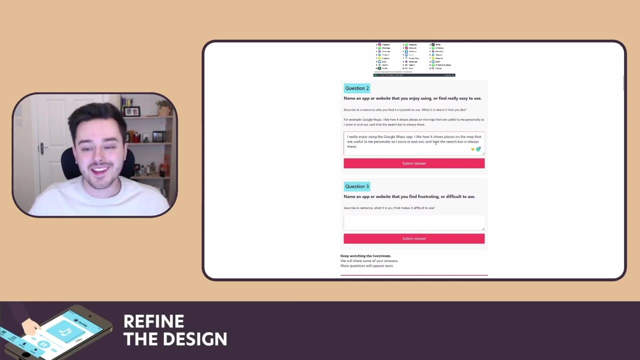 You want to mention and talk about what makes an app easy to use, what for those starting to consider using computer software apps and what makes it fun and interesting to use in teams, for example, Question 2. So, moving on to question 2, we're asked to name an app or website that 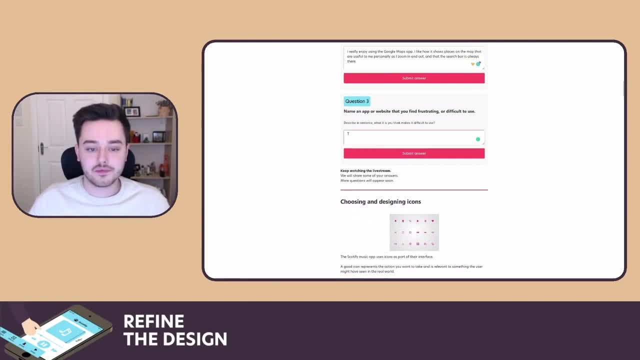 we enjoy using or find really easy to use. Our example answer here is: I really enjoy using the Google maps app. I like how it shows places and the map ads are really useful to me. difficult to use again, our answer here is: i don't want using the amazon app as the button. 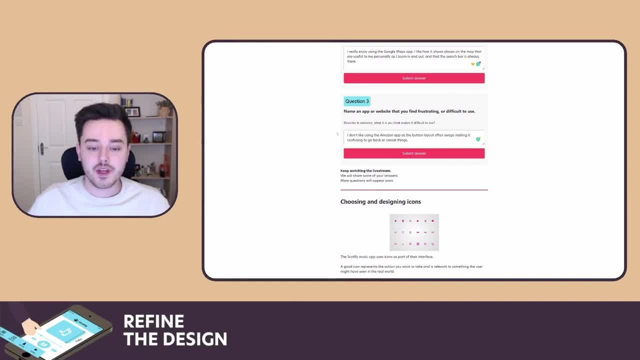 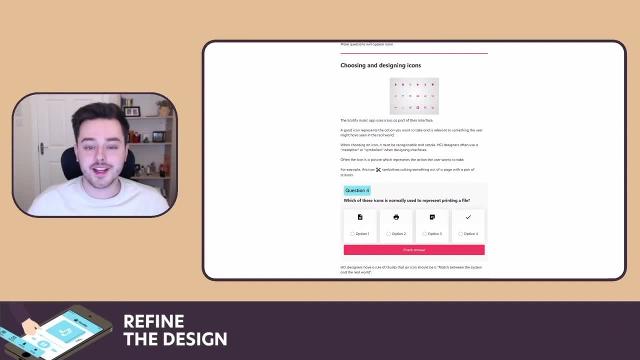 they often swaps, make it confusing to go back or cancel things. so, again, that's the answer. so now we're entering the choosing and deciding icon section. the scott app makes use of icons as part of their interface. a good icon represents the action you want to take and is relevant to something user may have seen in the real world. 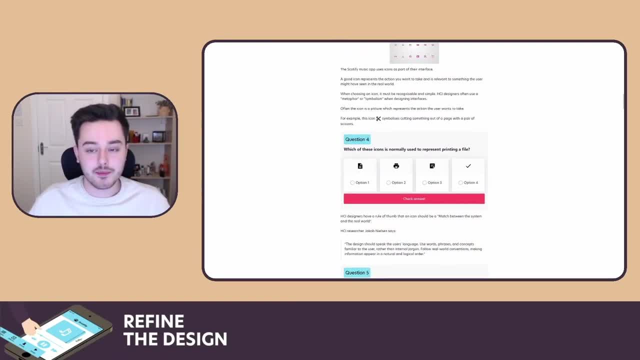 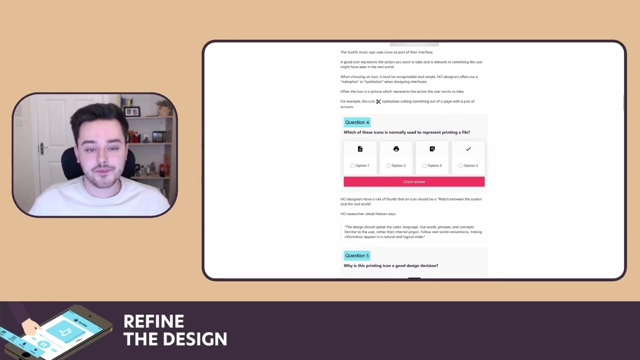 when choosing an icon, it must be recognizable and simple. each design designers often use a metaphor or symbolism when designing interfaces, often the pictures of the icons. a picture and represents the action the user wants to take. so example: here is a pair of scissors, if it's cutting out something out of the page. so we're going to question four: which of these icons is? 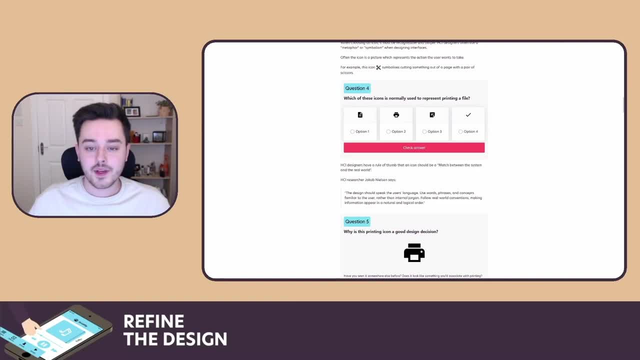 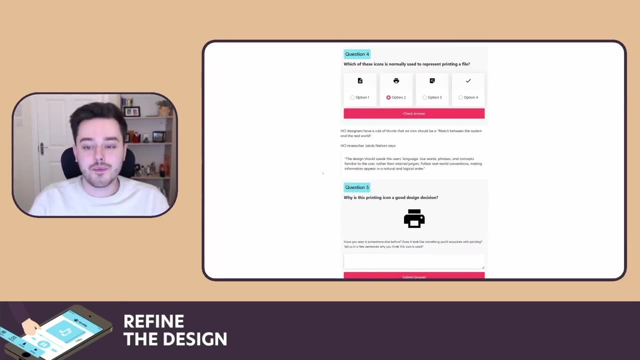 normally used in representing printing a file. so i've definitely seen option two before, and what the question is asking us is: what do we think? so i think it's option two. take answer to hate. designers all have a rule of thumb: the eye coaching. match between system and 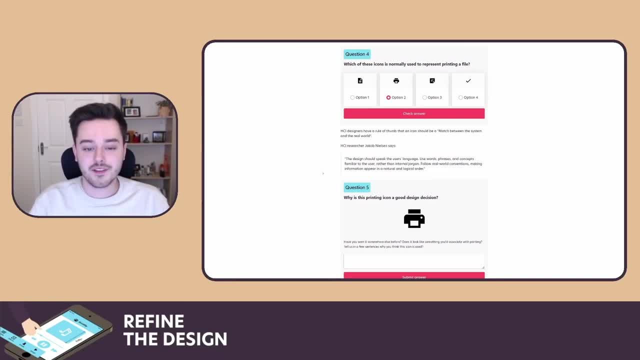 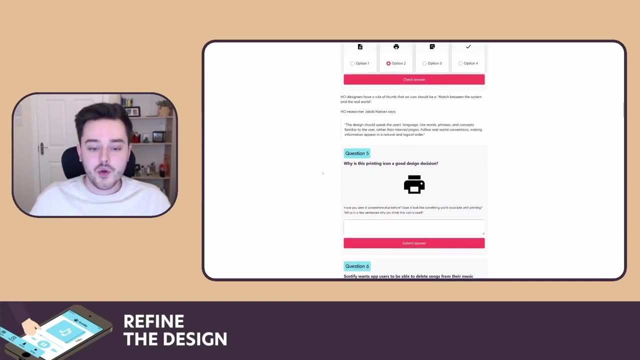 real world. there's a famous hci research called jacob nielsen and he says that his language should speak to users. use words, phrases and concepts related to the user rather than internal jargon. follow real world conventions making information appear in an actual logical order. moving on to question five, 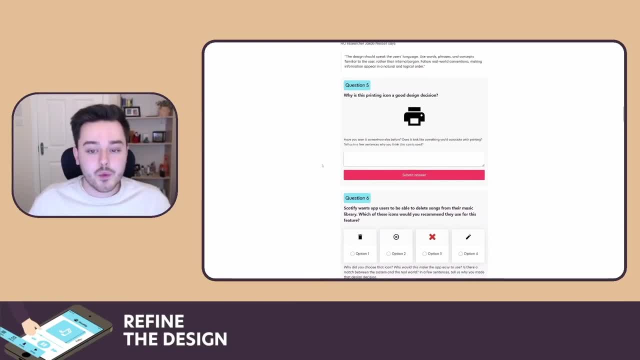 why is this printing icon a good design decision? have we seen it somewhere else before? so it looks something you'd associate with printing. so tell us a few sentences why this icon is used. so our example answer here is: the printing icon is a good design decision because it looks like a real 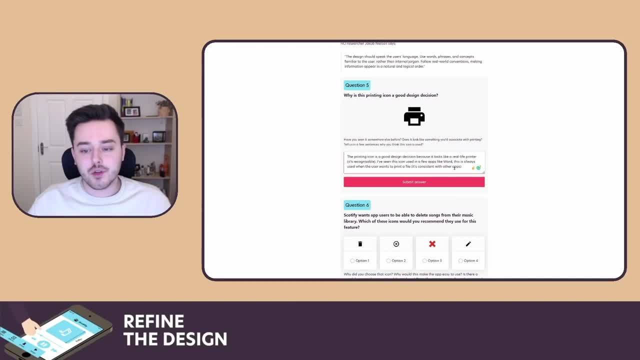 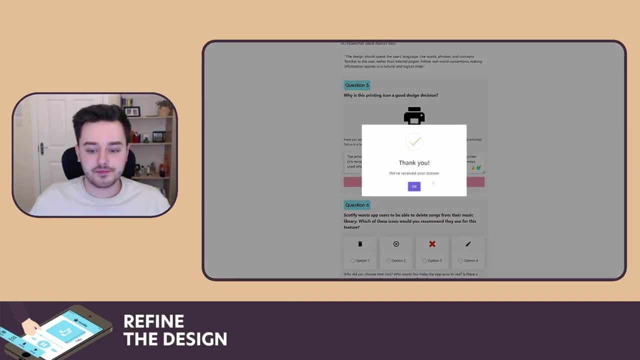 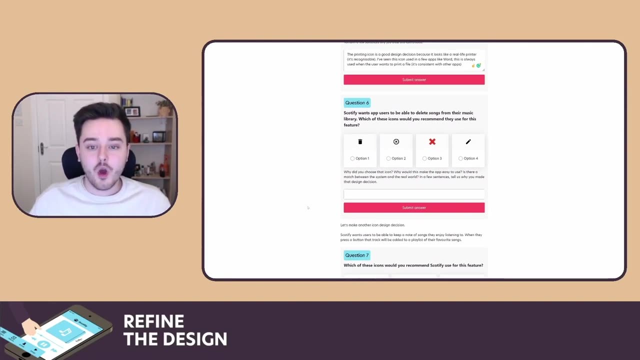 life printer. it's recognizable. i've seen this icon used on a few apps like word. i always use when the printer, when user wants to print a file, so it's consistent with other apps in question. six: scott fight wants abusers to delete songs from the music library. which of these icons? 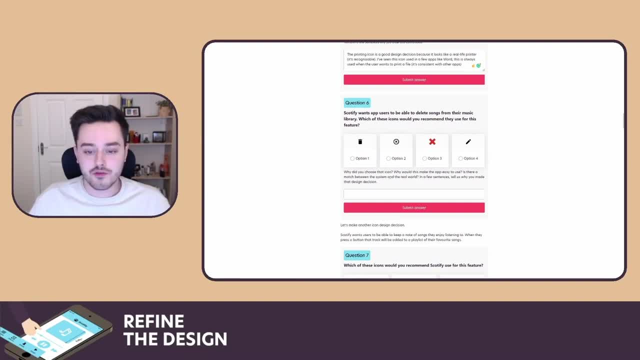 would you recommend they use for this feature? so a few options to choose from here. option two and three are very similar, showing some cross icons. option four is definitely more of an edit or pencil icon. i'm going to choose option one, going to look like a bin again. our example reading here is i: 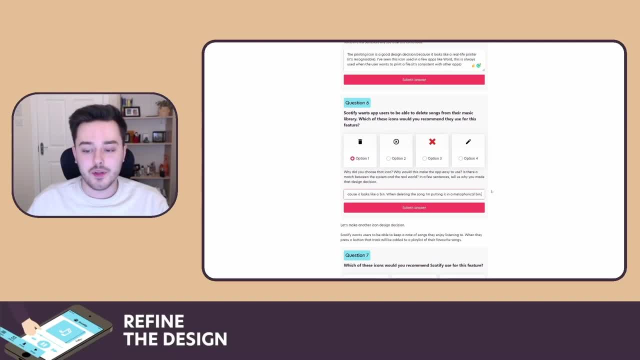 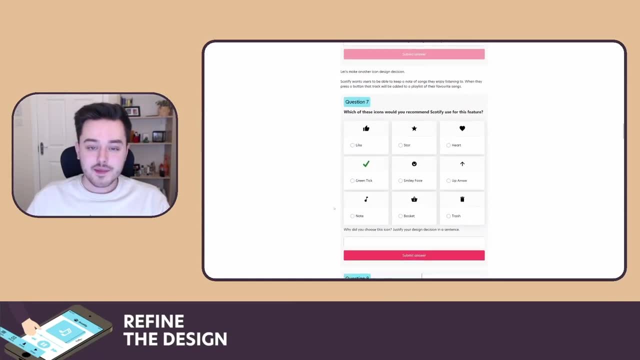 chose the first icon because it looks like a bin. indeed, in a song i'm putting it into a metaphorical bin. let's look at other icon design decision scott. if i want users able to keep a note of the songs they enjoy listening to, when they press a button, that track will be added to a playlist of our favorite. 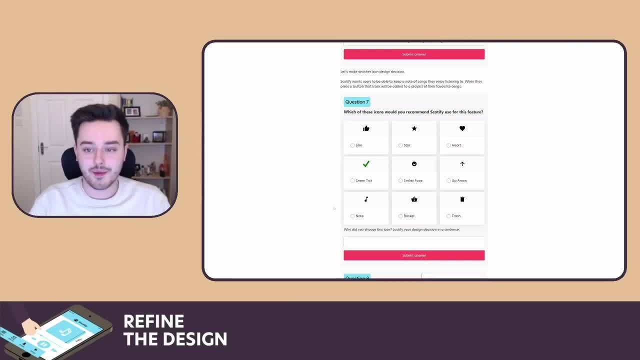 songs. question seven: which of these icons would you recommend scottify use for this feature? so the bottom row for me is definitely not icons i would use i could. the second row here is a bit better, but definitely the ones in the top and i'm going to choose a heart because i've seen that before. 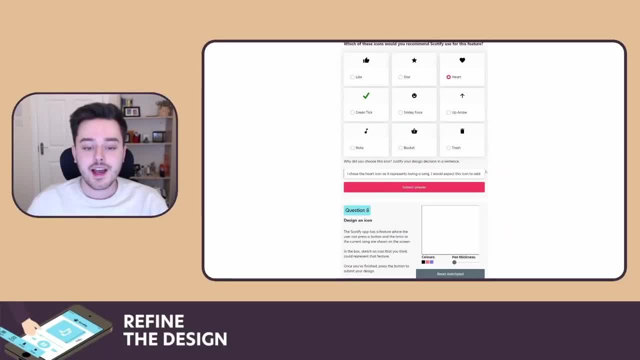 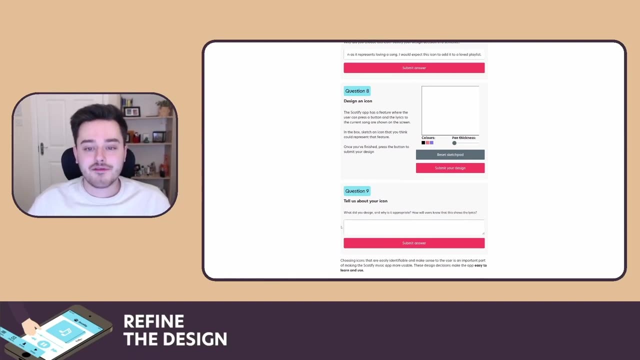 and our example really, really weird is i chose the heart icon as it represents loveliness song of expects icon to add it to a loved playlist. obviously, designing an icon, it's got fit up as a feature where the user can press a button and the lyrics of correct release song are showing on the screen in the text box sketching icon that you 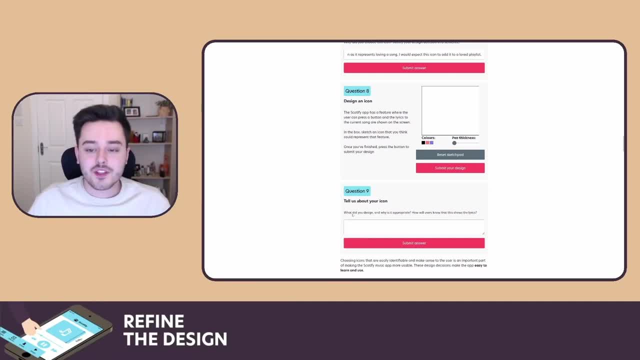 think represents this feature. so if question is quite cool, we get to draw our own icon, so i will. so here we have our color control and our pen thickness. so, to get started, I'm going to change it to blue, add a little bit of thickness, and I'm going to add some lines representing lyrics. 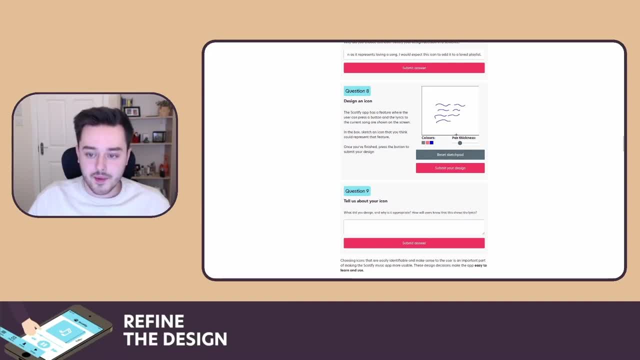 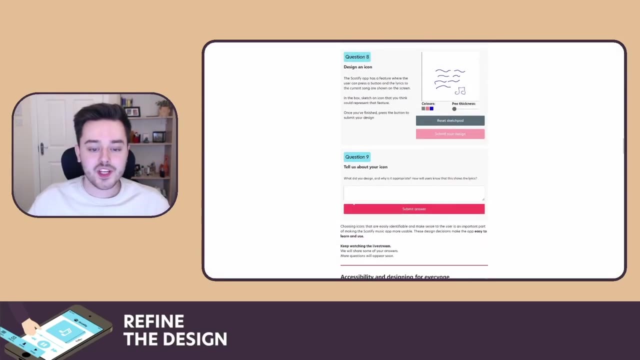 then I'm going to change it back to black here and I might draw show back to some music. so that's some of that design. and now in question 9 we're being asked to describe our icon and our example. reasoning here is: I used a musical note to show some music. 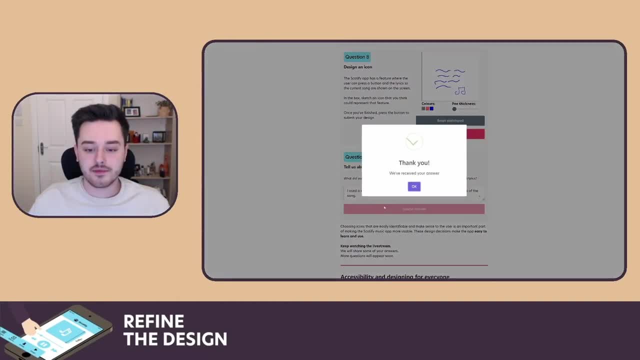 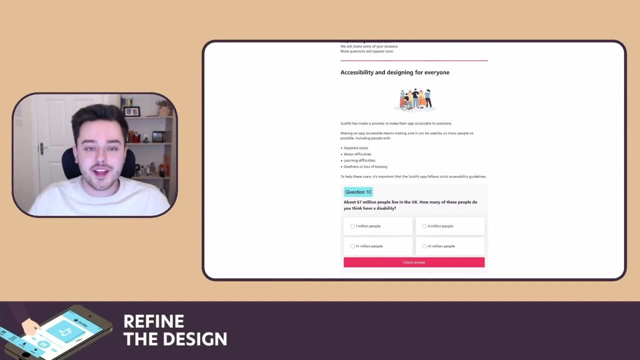 and lines representing the lyrics of the song. so that's sitting that across. and that brings us into the end of the iconography section. our next section is accessibility and design for everyone. so Scottifies made a promise to make the app accessible to everyone. basically, making the app accessible means making sure it can be used to as many people as possible. 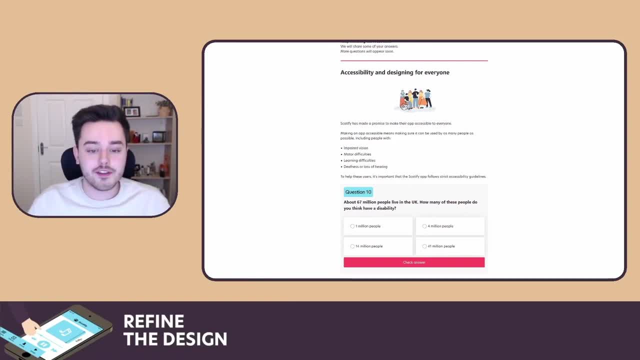 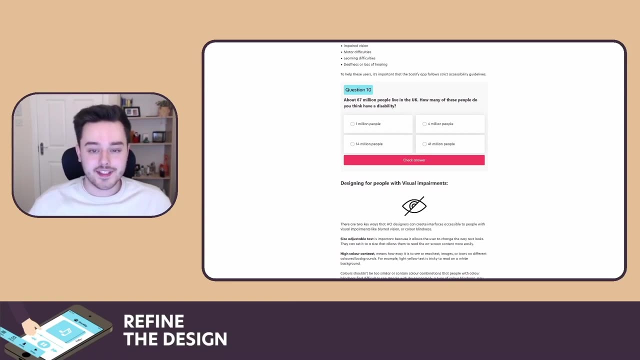 and that includes people with impaired vision, motor difficulties, learning difficulties, and deafness and loss of hearing. to help these users, it's important that Scottify app follows strict accessibility guidelines. question 10: around 67 million people live in the UK. how many of these people do we think have a disability? 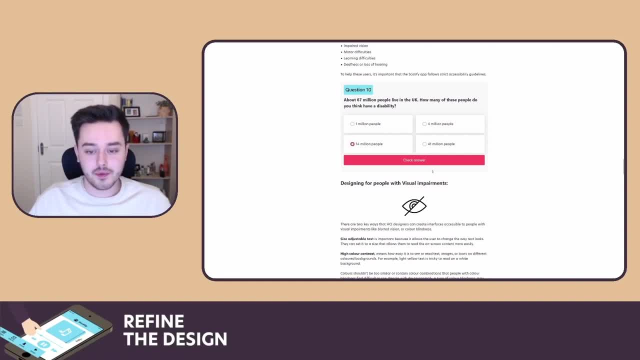 there's a few options we should choose, but I'm going to select 14 million people and check that answer. so that's a great answer and we can see the bottom of a source button so that the learners can click on to see where the information came from. 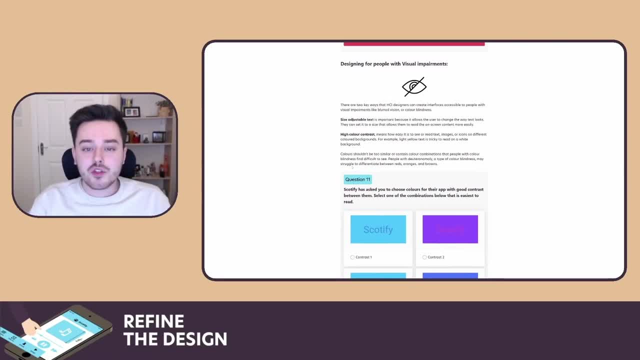 so designing for people with visual impairments. there are two key ways that hate site designers can create interfaces accessible to people with visual impairments, like blurred vision or colour blindness, and these are size adjustable text. this is important because it allows users to change the way text looks. 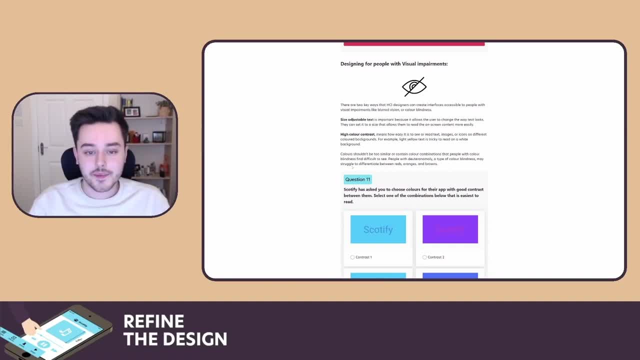 they can set it to a size that allows them to read the on-screen content more easily. another way is a high colour contrast, meaning how easy it is to see or read text, images or icons on different colour backgrounds. for example, light yellow is very tricky to read on white backgrounds. 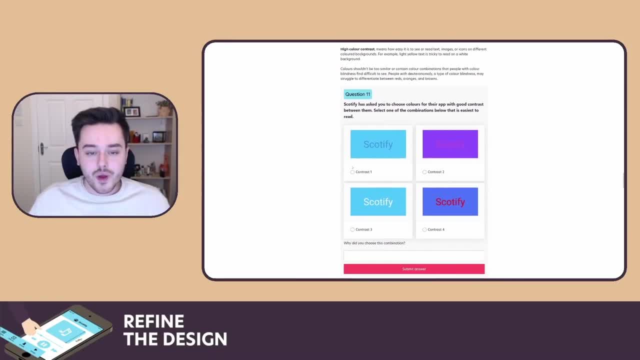 this is very important to people with colour blindness. so question 11: Scottify has asked you to choose colours for their app to create contrast between them. if you dislike the one combination below, it's easiest to read, so straight away. I find contrast 2 very difficult to read. 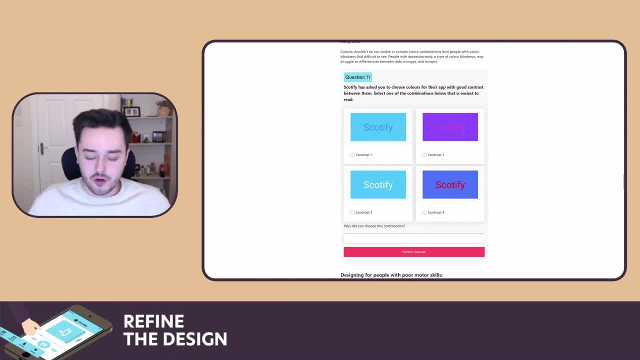 and contrast 4 hurts my eyes, so I'm more drawn to contrast 1 and contrast 3. I do think that contrast 3 is the most easy to read, so I'll select that one and another. example reasoning here is: I chose a blue and white colour contrast. 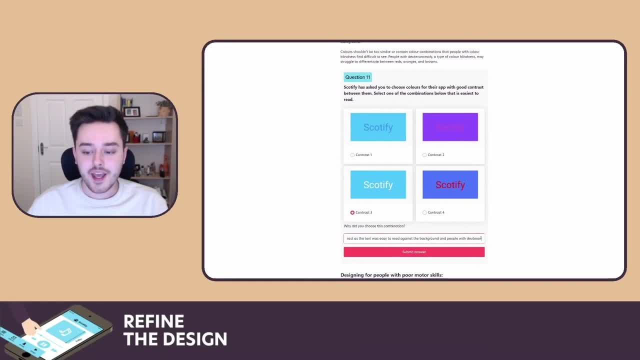 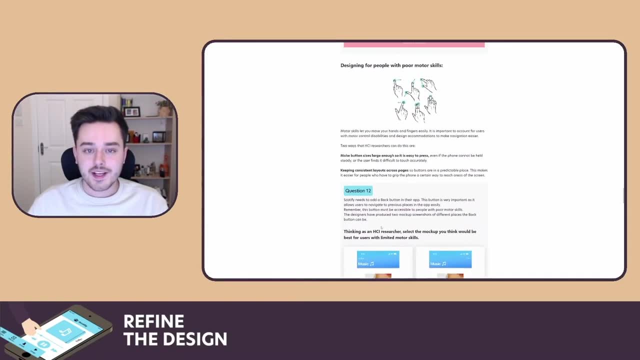 but the text was easy to read against the background and people with colour blindness will be able to read it as well. so that's my answer: designing for people with poor motor skills. so, motor skills, let you move your hand and fingers easily. it's important to account for users with motor control disabilities. 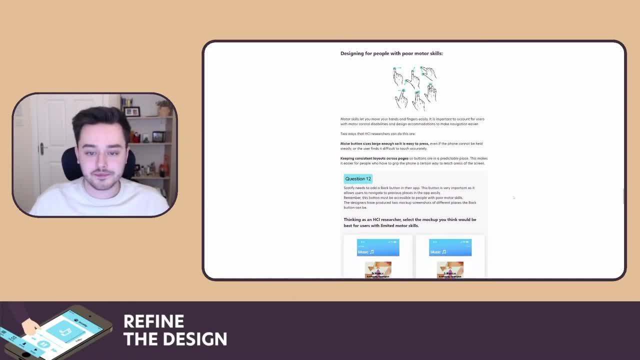 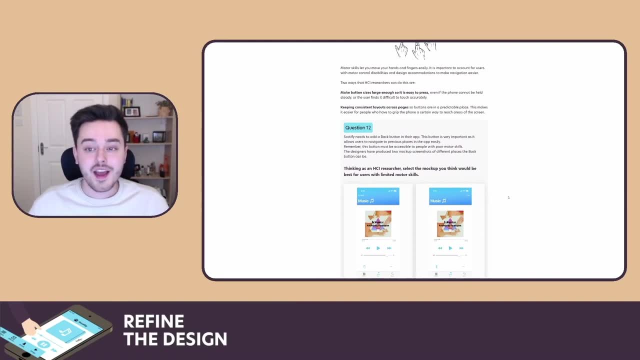 and disabilities to make the navigation easier. there are two ways that heat side signers can do this: they make button sizes large enough for it to be easy to press, even if the phone cannot be held steady or the user is kind of difficult to touch accurately, and keeping consistent layouts across pages. 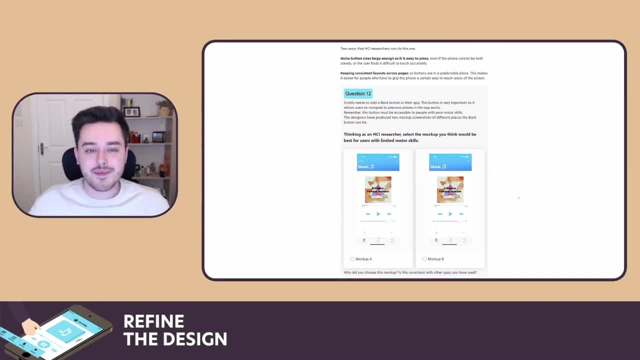 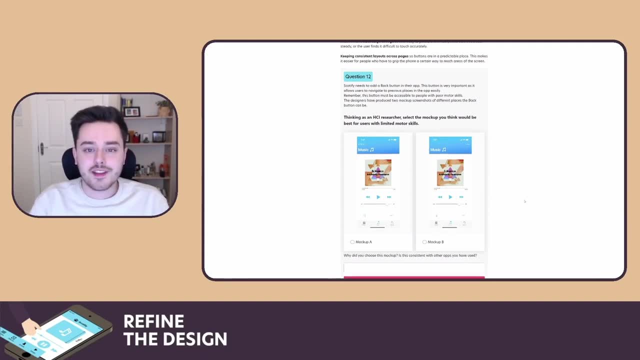 so buttons stay up to its own place. this makes it easier for people who have to grip the phone in a certain way to reach areas of the screen. so in question 12, Scottify needs to add a back button to your app. this button is very important. 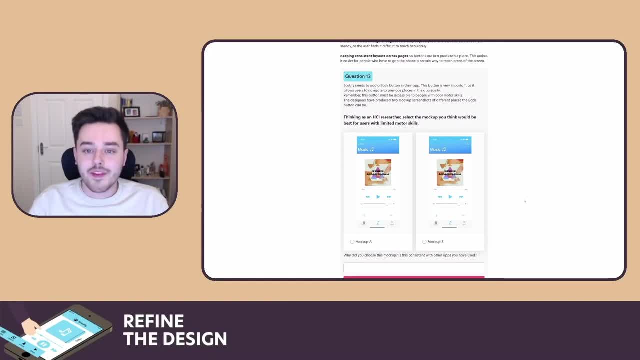 as it allows users to navigate to previous places in the app. as a member of this must be accessible to people with poor motor skills, so the designers have produced two mockup screenshots and they're replacing the back button, and I think because I'm a heat side designer- 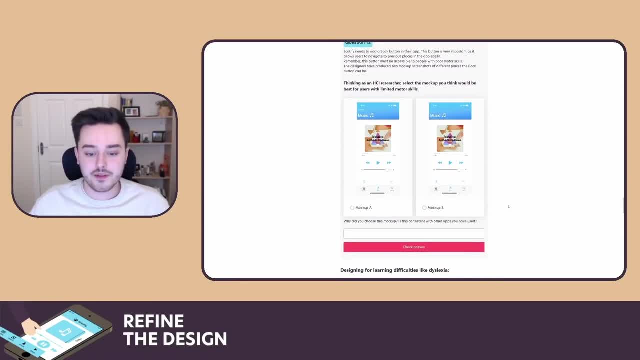 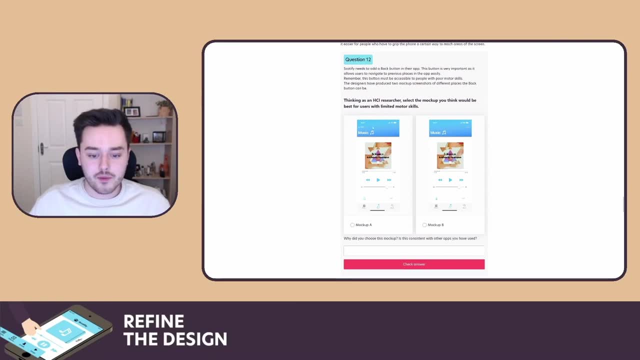 we just like the mockup B thing the best for people with limited motor skills. so in mockup A I can see the back button is in the top left and it's in the right in mockup B, but there's much bigger on the mockup A. 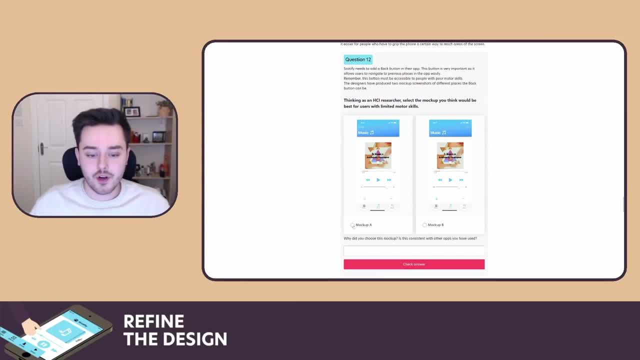 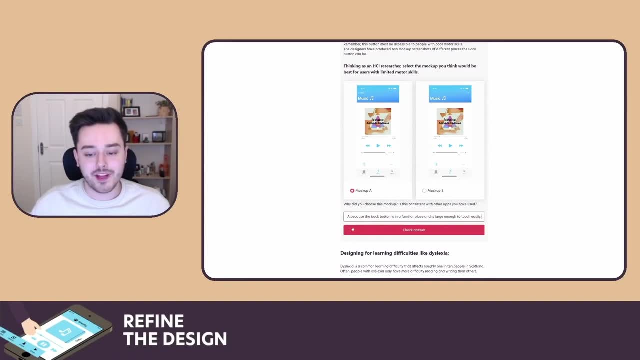 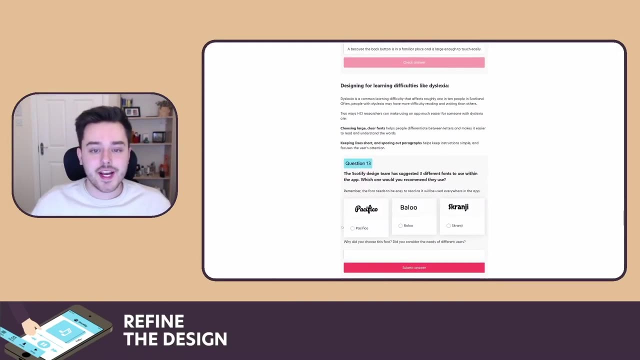 and I've definitely seen the back button not used in the left before, so I'm going to select mockup A again and our example reason here is: I chose A because the back button is a familiar place and large enough to touch easily. so, moving on designing for people with learning difficulties like dyslexia. 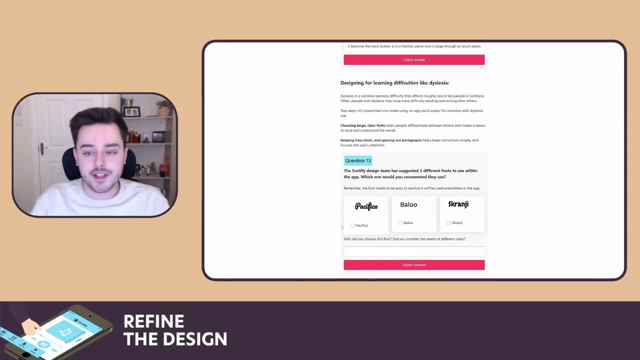 so dyslexia is a common learning difficulty that affects roughly one in ten people in Scotland, and often people with dyslexia may have more difficulty reading and writing than others. once again, there are two ways. heat side researchers can make your app much easier for someone who has dyslexia. 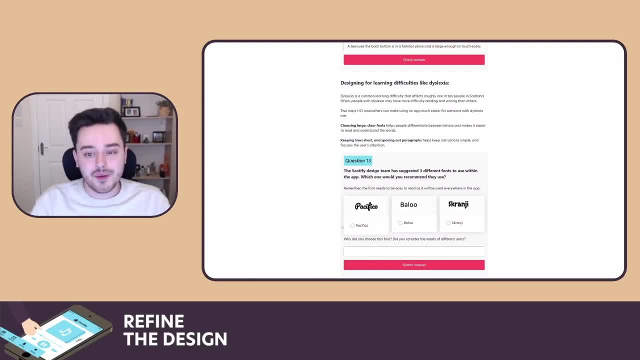 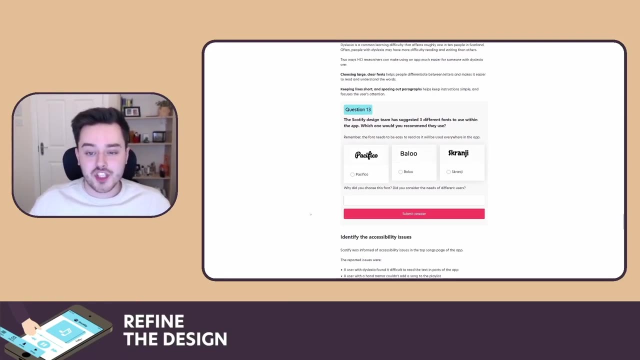 and they are choosing large, clear fonts. it helps by: helps people differentiate between letters and makes it easier to read and understand the words and keep your learning short in spacing and paragraphs helps keep instructions simple and focuses user attention. question 13: scottify design team would suggest you. 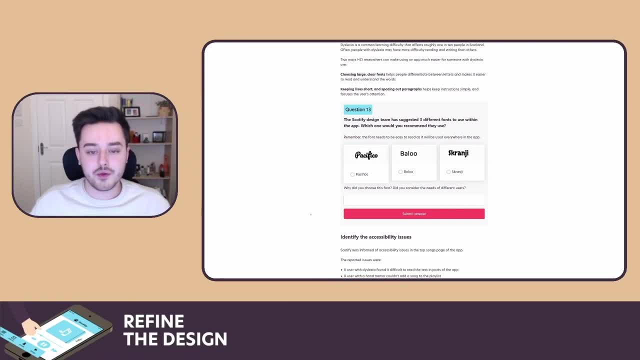 seek three different fonts to use in the app. which one would we recommend that they use? you need to remember this font will be easy to, needs to be easy to read as it will be used everywhere in the app. so we have the font here: pacifico, blue and scrangie. 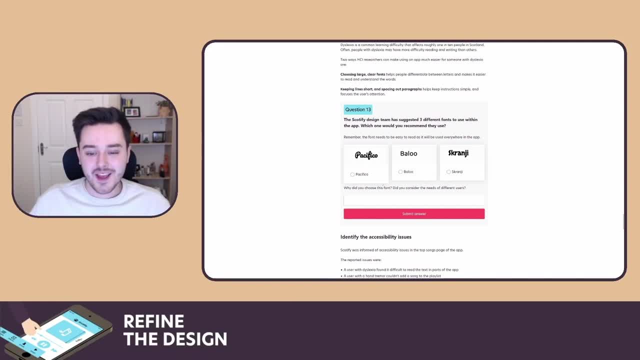 I really like pacifico because I just think it's quite fancy and nice. but blue is definitely easiest for me, as I don't like this one at all. so let's take a look. and so our example reason here is: I would use the blue font as it's straightforward and easy to read. 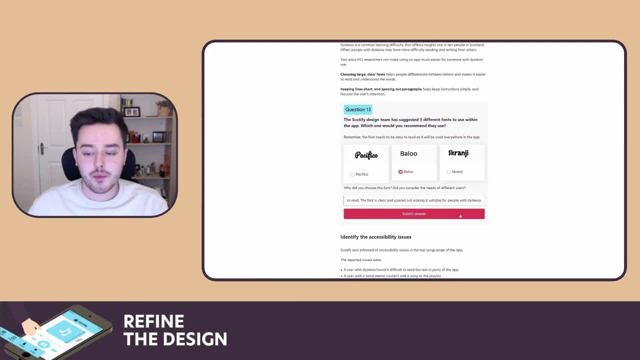 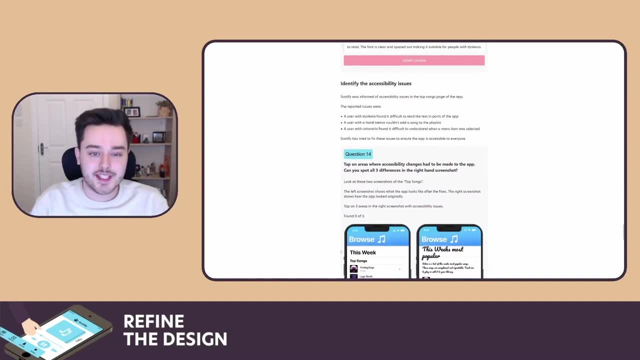 the font is clear and spaced out, making it suitable for people with dyslexia. now, as I did find some accessibility issues, scottify was informed of accessibility issues in the top songs page of their app. major reported issues were: a user of dyslexia found it difficult to read the text in certain parts of the app. 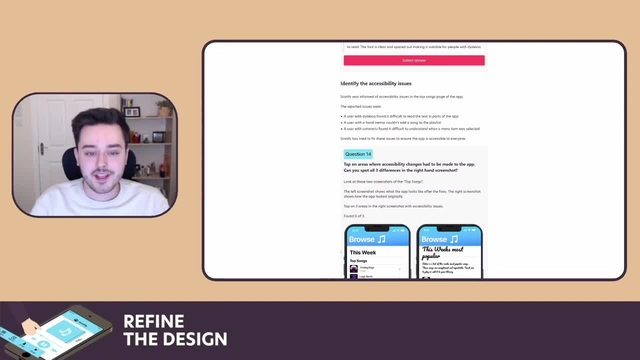 a user of a hand tremor couldn't add the song to a playlist and a user of cataracts found it difficult to understand when a menu item was selected. scottify said to try to fix these issues to ensure the app is accessible to everyone. 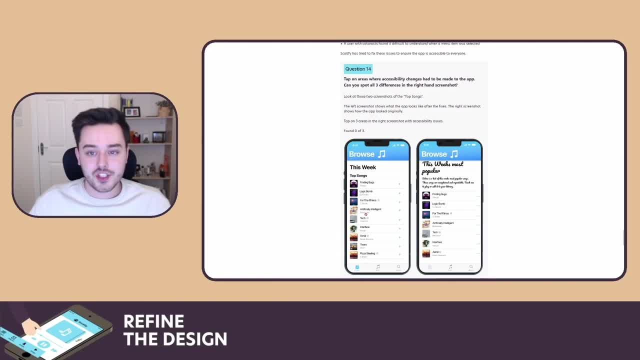 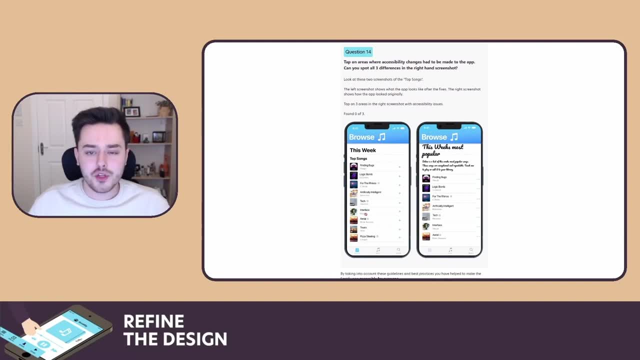 in question 14 tap on areas where accessibility changes had to be made to the app and can respond to all three differences in the right hand screenshot. so we can look at the two screenshots of the top songs page. the left screenshot shows the app how it looks after the fixes. 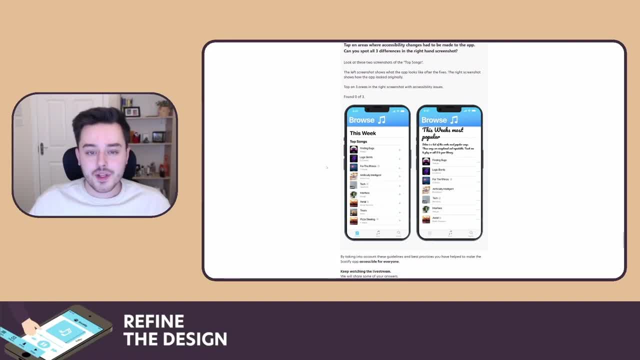 and the right screenshot shows how the app looked originally. we tap on three areas in the right screenshot of accessibility issues. so, looking at the right hand screenshot here, I definitely see one at the top here, this one, which is not very good, so let's click here. great, so that's pulled up, us finding an accessibility issue. 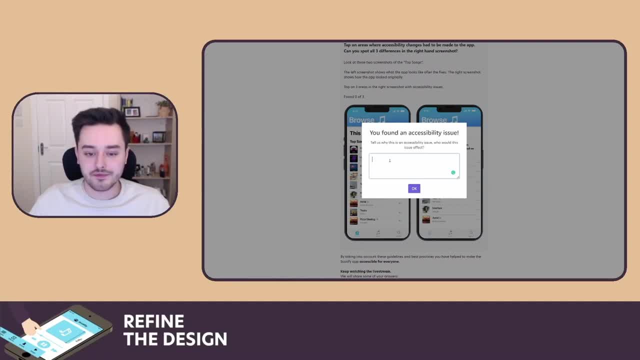 where we can type in our reasoning for why it's an accessibility issue, and our example reasoning here is: the font is difficult to read and will be unsuitable for people with dyslexia. so let's zoom that across and I've found one out of three. 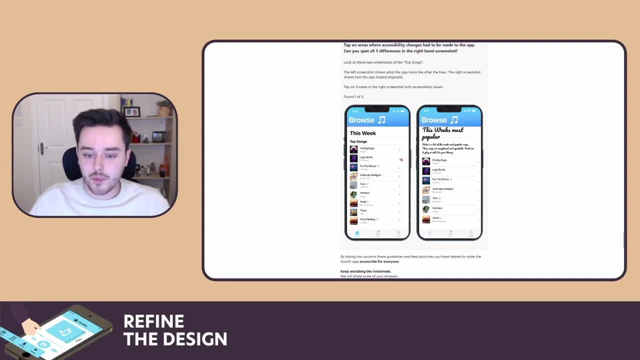 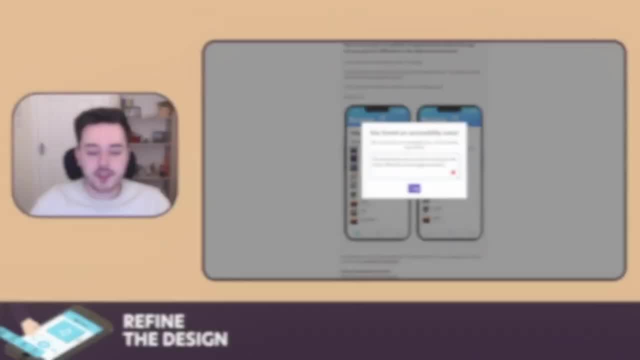 and there's definitely one here. so this bottom here is far too small compared to on the left hand side. so let's then put why we think it's the case, and our reasoning here is: the ad buttons are too small for people with most disabilities and they will struggle to press it. 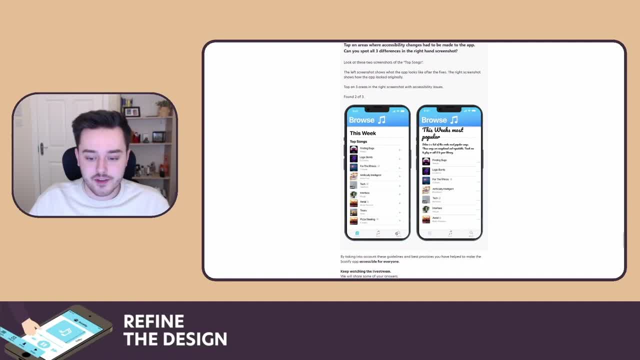 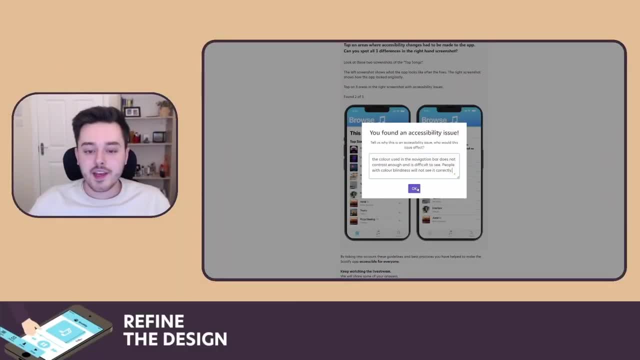 and our final one. I think this problem with contrast here is very different in these two, so let's click on this one. great, so that's entered. why, and our example reasoning here is: the color used in the navigation bar does not contrast enough and is difficult to see. 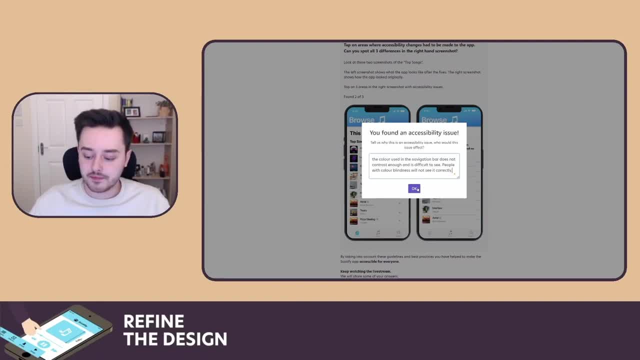 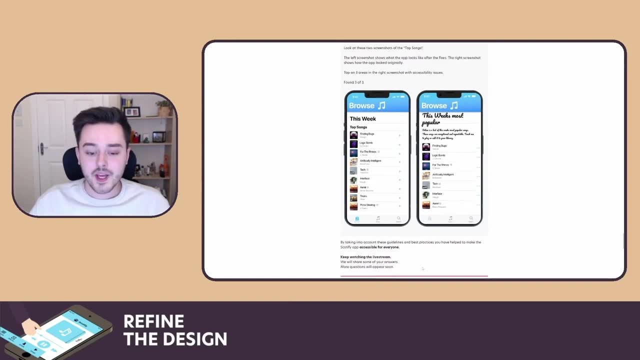 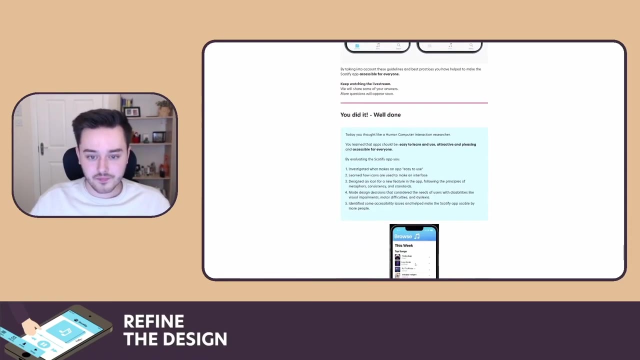 people of colorblindness will not see it correctly, so let's assume this one great. so that's found all three accessibility issues. by taking into account these guidelines and best practices, we've helped to make the scottify app accessible to everyone, and that's it. 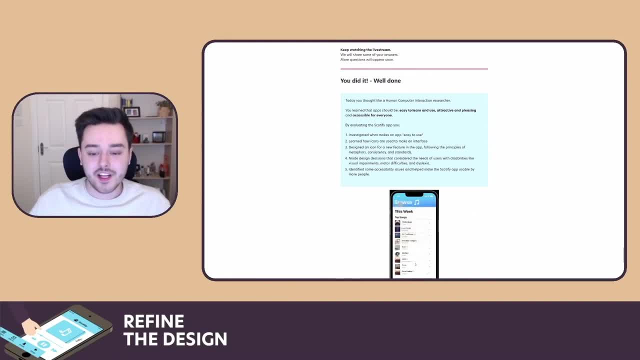 so we've come to the end of the refining design activity. learners can now see a mock-up of the finished scottify app after all their fixes. so thanks for listening to the walkthrough video today and have fun refining the design. thanks,